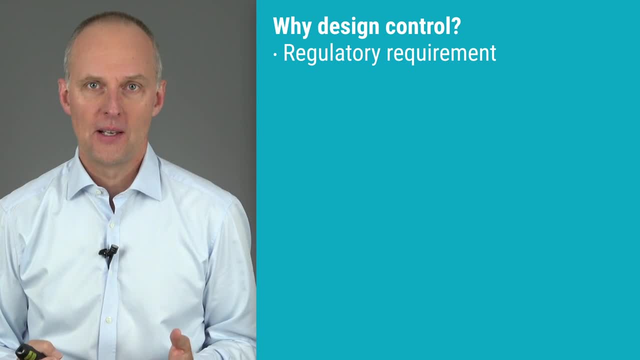 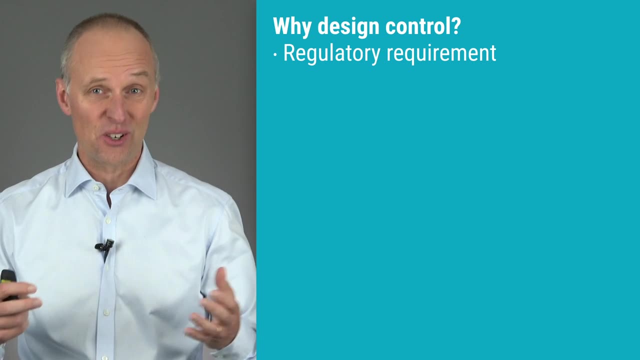 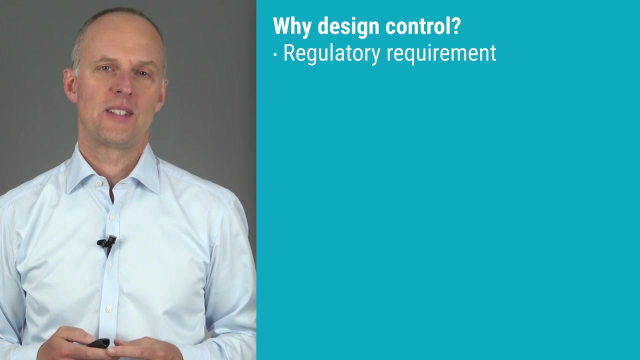 complying with design control requirements is a regulatory requirement. This is technically correct. but if someone tells you that you should work with design control only because it is a regulatory requirement, I think that person has overlooked something very important. Working according to design control requirements is an effective way of creating products that are not only safe. 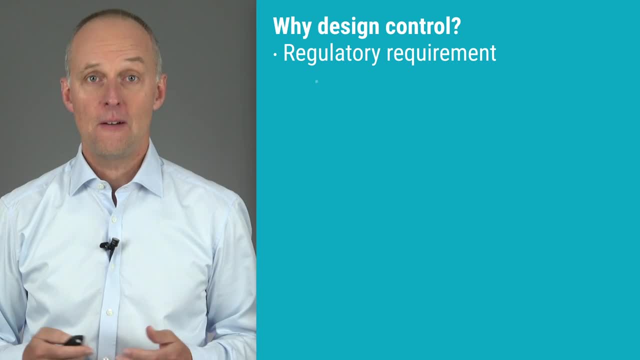 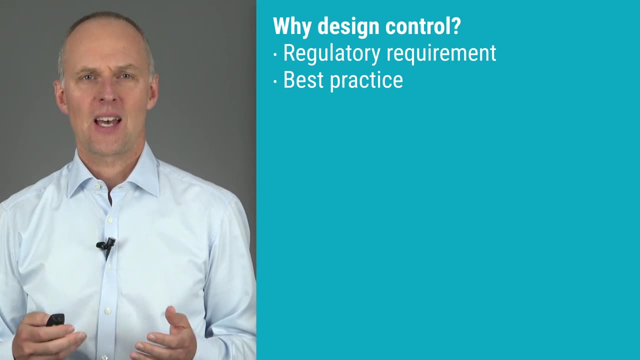 but that will also satisfy your customers' needs. In fact, most of the design control requirements represent best practices in developing new products, And if you look at companies from other industries where design control is not a requirement, you will find that companies are working according to these requirements. 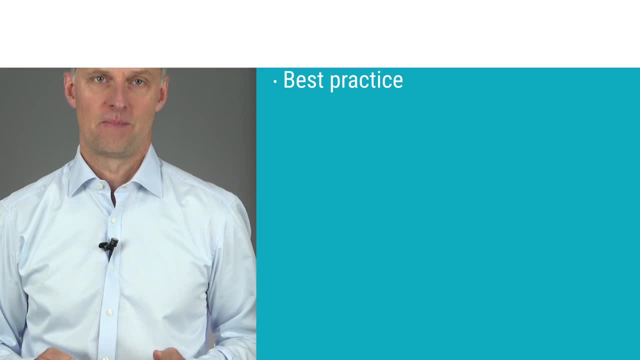 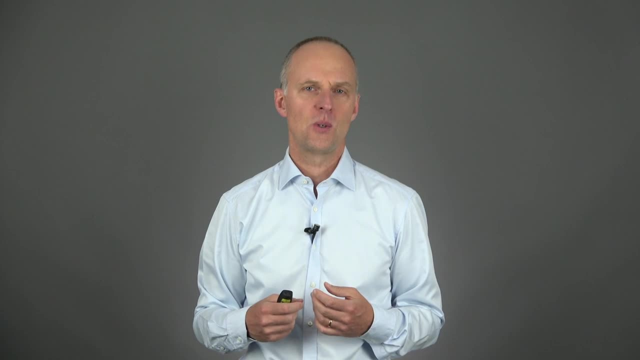 And that's because they see the value in it. We can therefore conclude that learning about design control is not only about doing things in a certain way to gain access to the US and European markets, but it is to learn how to be successful in developing products that meet your customers' needs. 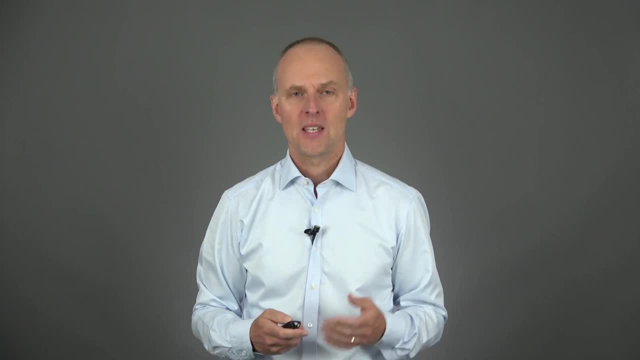 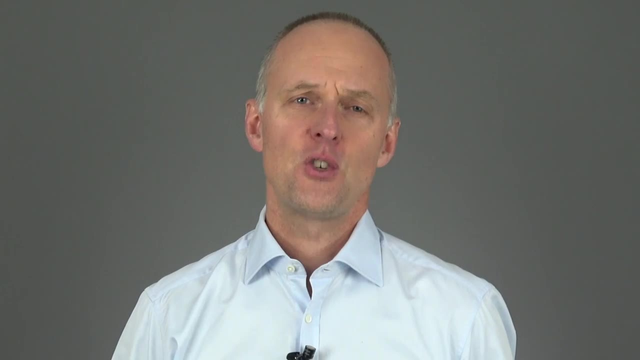 And that can never be wrong, can it? Keep that in mind during this course? What you are learning are best practices and not only regulatory requirements. So before getting back to what design control is in more detail, a few words of caution. We are now. 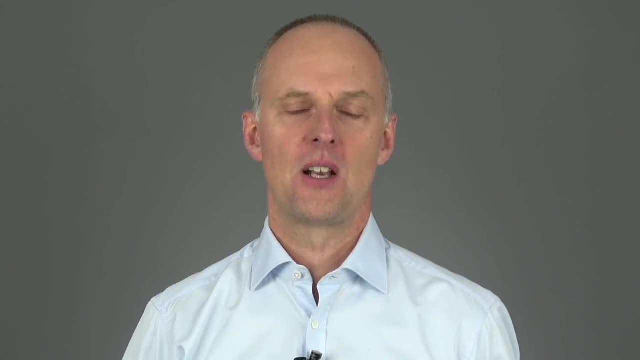 going to run straight into a lot of three-letter acronyms and nerdy standard names and numbers. Don't let them scare you At this time. you don't need to know them all by heart, but you should recognize them when you see them or hear about them. 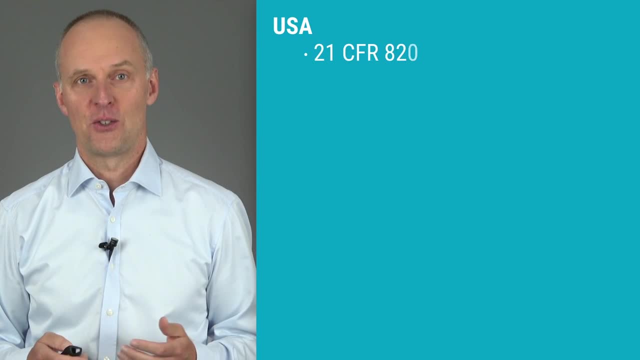 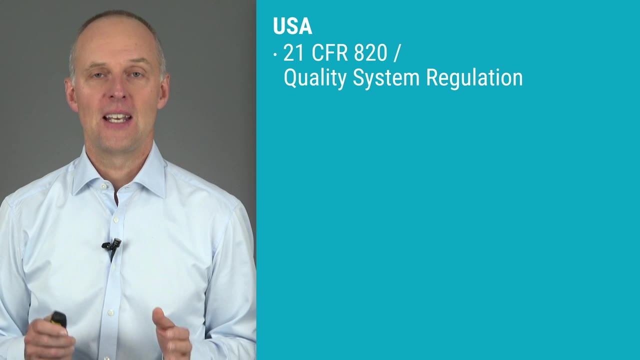 Design control is the area of requirements from the US Quality System Regulation, or QSR, that apply to the design and development of a product. To be even more specific, it is subpart C of the QSR and clause 82030 that is called design control. 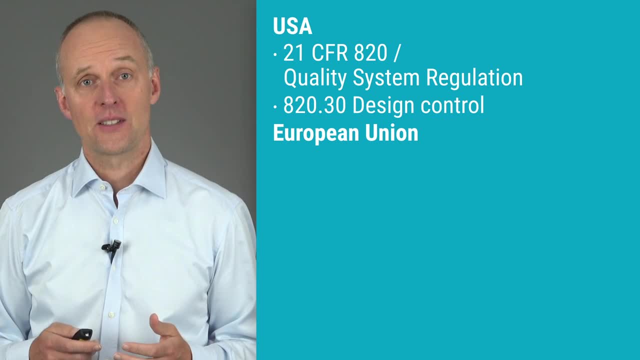 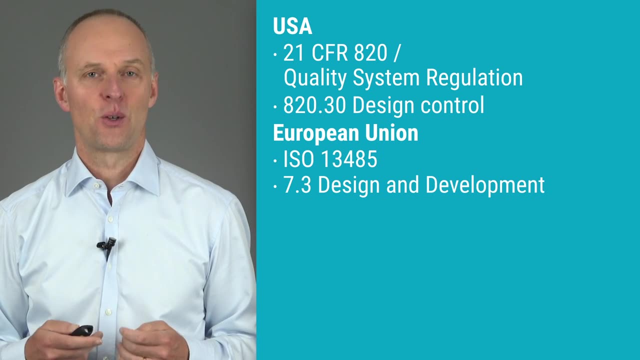 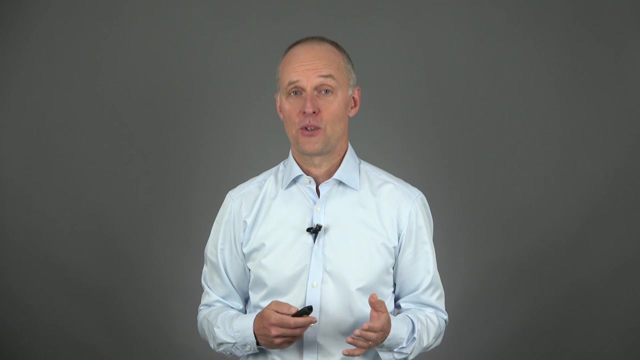 The corresponding term for design control in a European context would be design and development, and the requirements relating to that area can be found in section 7.3 of the ISO 13485 standard. You might have heard about the new medical device regulation that will soon be enforced in Europe. 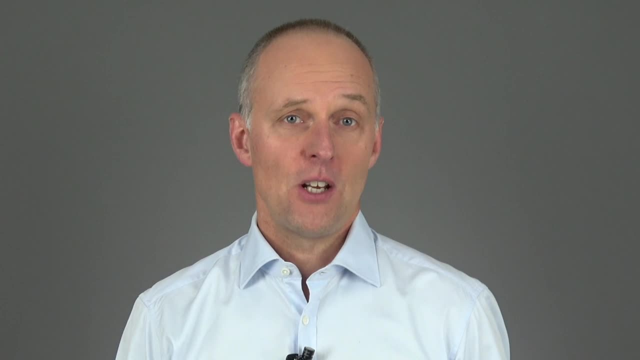 getting back to that later on during this course. As you may know, there are a lot of requirements that apply to medical device manufacturers. To be honest, they can appear as somewhat overwhelming at times. Luckily, the requirements we will be looking at during this course will take you really far. 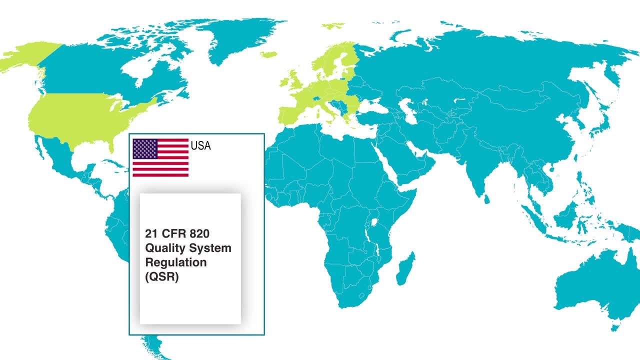 Let's break them down. In the US, there is a regulation called 21 CFR 820, or Quality System Regulation, or just short QSR, which is maybe the easiest thing to remember. That establishes requirements for manufacturers that want to sell their products in the US market. 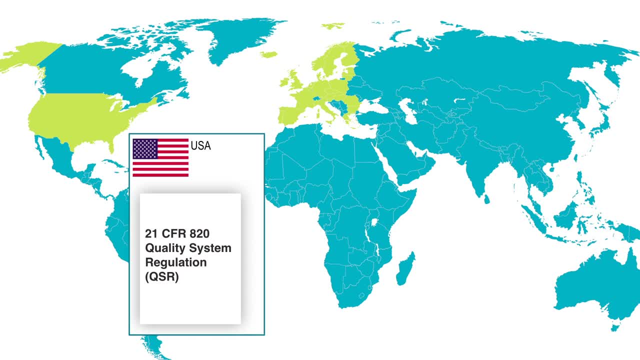 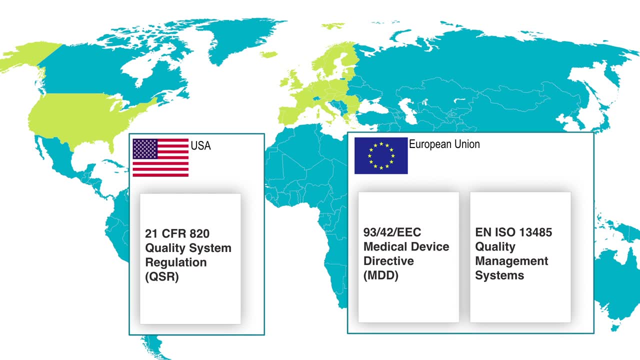 This is the regulation in which you will find the subpart on design control. In the European Union, we currently have 3 directives that cover regular medical devices, active implantable medical devices and in vitro diagnostic medical devices. These directives share a lot of requirements. 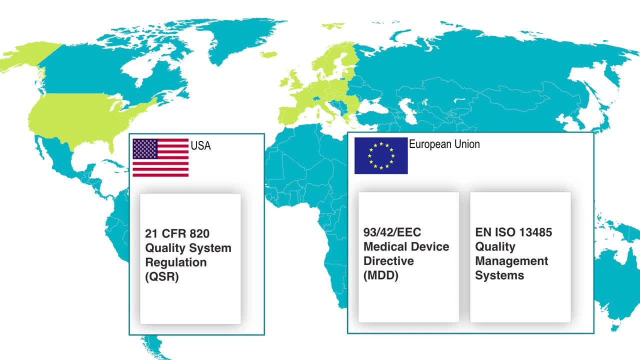 So currently on this course, we will focus on requirements that apply to medical devices. Thank you for all of the revelations we got in this Brigade to the directives just mentioned, most manufacturers would also comply with the requirements of the ISO 13485 standard on quality management systems, The reason for that being that 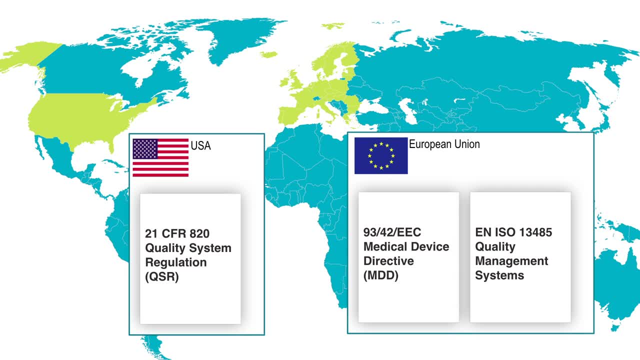 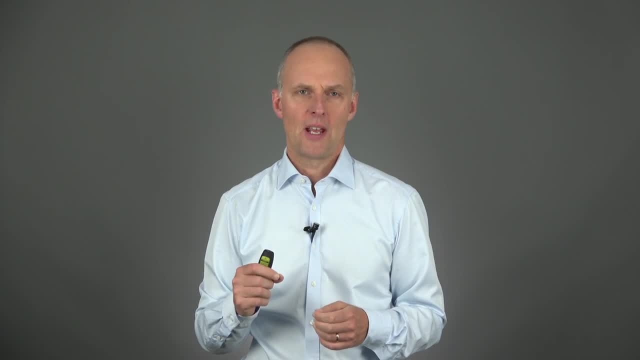 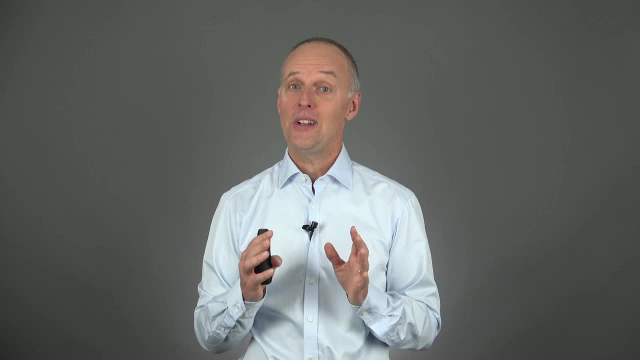 the standard contains more detailed requirements on the quality management system than the medical device directive does. Even though product development should be done more or less the same way all over the world, there is one caveat: Submissions for product approvals and reviews of your technical documentation will differ a lot from one country to another. but rest assured. 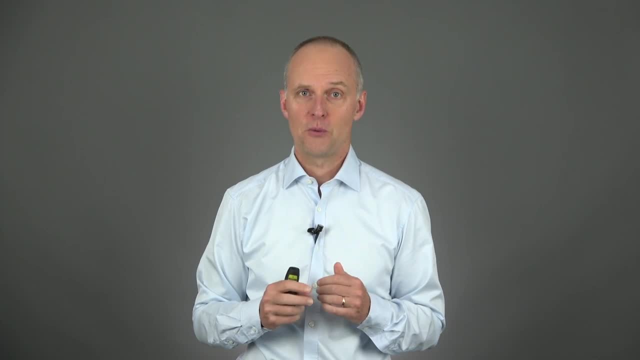 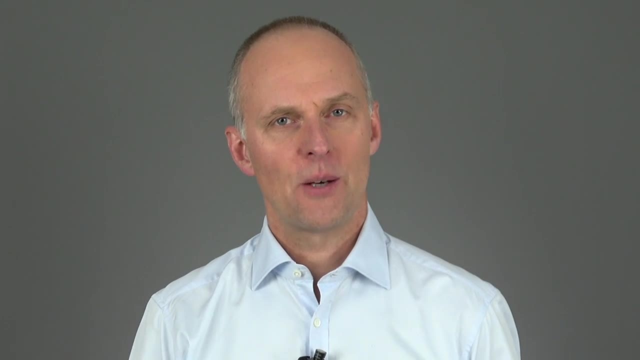 implementing the concept of this course will suffice for most medical device markets in the world. when it comes to how you actually do the product development, What do you think? Is there anyone out there that checks that medical device companies are doing things the way they should? 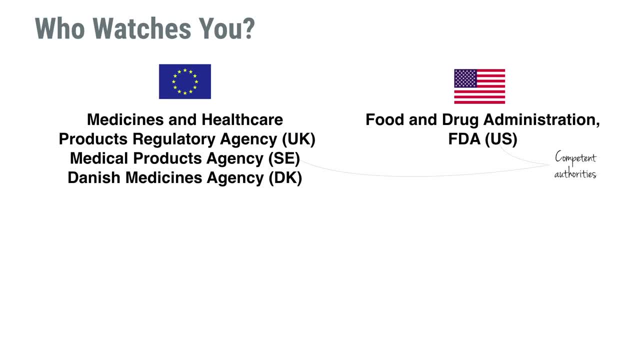 Yes, there is. In the EU, each country has a supervising government entity for medical devices. In the United Kingdom that would be the MHRA. in Sweden it would be the Medical Products Agency. in Denmark it would be the Danish Medicines.